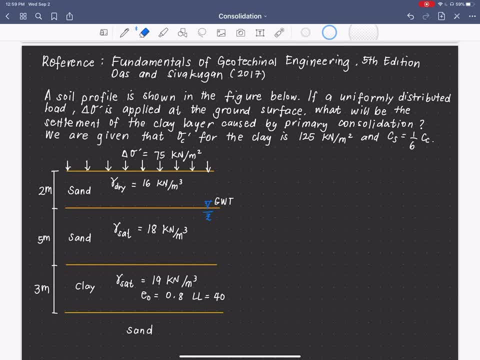 We have a specific formula for normally consolidated clay and for over-consolidated clay, So the first thing that we need to check is whether the soil is normally consolidated or over-consolidated, And the given parameters are delta, sigma and sigma sub c. 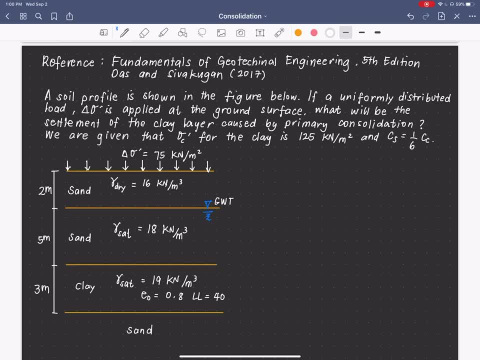 Now to check if it's normally consolidated, we have to calculate the effective stress at the average effective stress at the center of the clay layer. So here, at this point, So to begin, let us solve or calculate the effective stress at the center of the clay layer. so if we start from the ground surface, the formula is gamma sub. 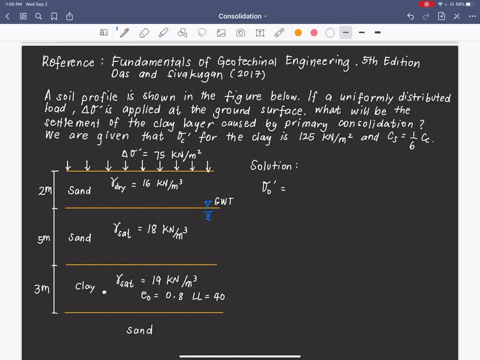 D, or the unit weight of the soil multiplied by the depth. so the first layer is sand. so we have gamma dry of sand multiplied by the depth of sand, which is two meters. plus the second layer of sand is already submerged, so we have to multiply the gamma submerged or the unit to 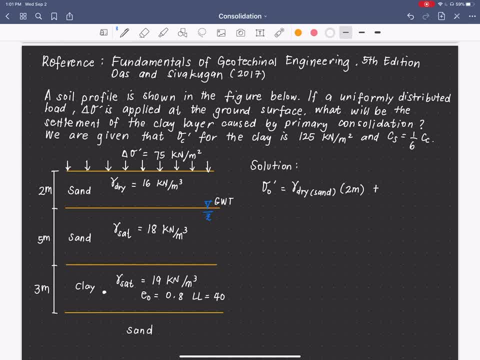 its submerged by its depth of five meters and the submersion it we can be calculated using gamma saturated of sand minus gamma water x. the depth of five meters plus at the center of the clay layer, the depth is 1.5 and the submission it weight of the clay. 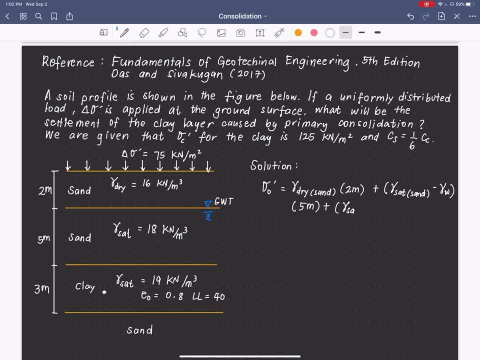 layer is gamma sat of clay minus gamma water, multiplied by half of 3 meters, which is 1.5 meters. so let's substitute the given values. the dry unit weight of sand is 16 kilonewton per cubic meter. this is to be multiplied by 2 meters. 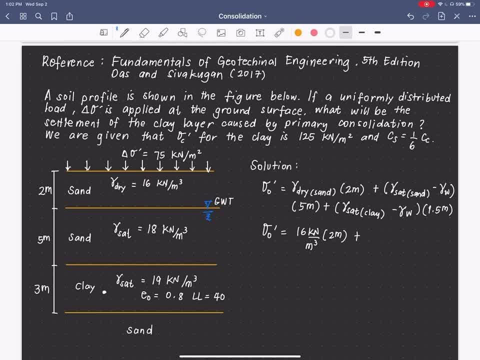 plus the saturated unit weight of sand, which is 18 minus the unit weight of water: 9.81. this is in kilonewton per cubic meter, cubic meter multiplied by the depth of 5 meters. then plus the saturated unit weight of clay, which is 19 minus the unit weight of water, 9.81. again, this is 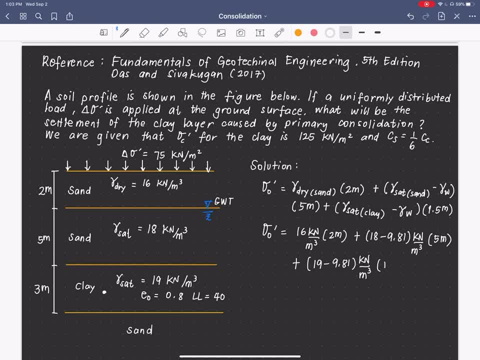 in kilo Newton per cubic meter, multiplied by 1.5 meter step of clay, and when you try to calculate and simplify, we'll get an answer of 86.74 kilo Newton per meter step of clay. and when you try to calculate and simplify, we'll get an answer of 86.74 kilo Newton per. 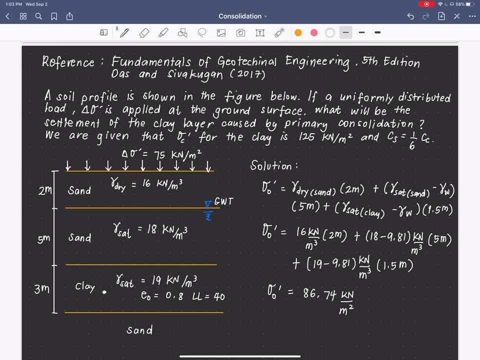 square meter. So that is the effective stress at the center or the middle of the clay layer. So let us compare the preconsolidation stress to the effective stress, Since our given preconsolidation pressure sigma sub c prime is 125. 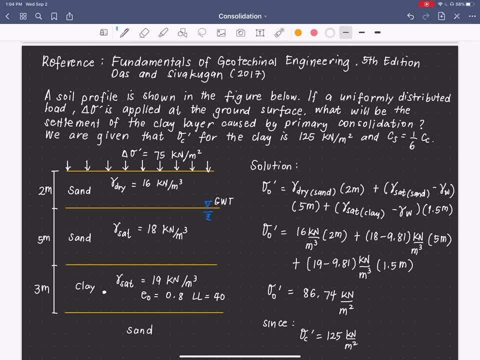 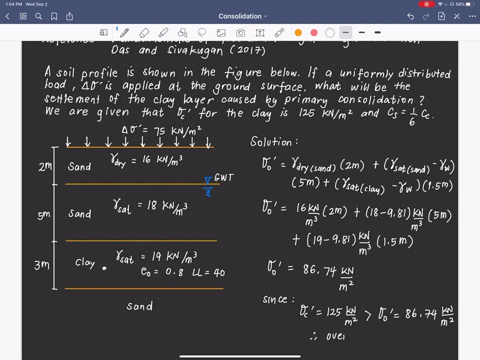 kilonewton per square meter. this is obviously greater than the overburden pressure or the effective stress of sigma sub c prime: 86.74 kilonewton per square meter. therefore, our clay is over consolidated clay, in which case we're going to use the formula developed for the over. 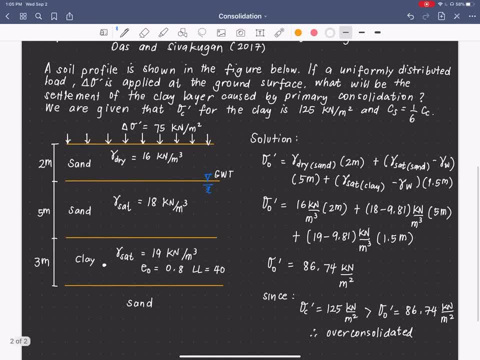 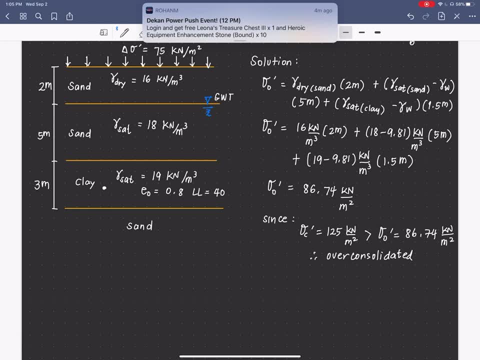 consolidated clay and, if you remember, we have two formulas or equations for over consolidated. before we use this formula we have to check first some conditions. we need to compare the sum of the overburden pressure and the surcharge with the pre consolidation pressure, so we have to know if it is greater than. 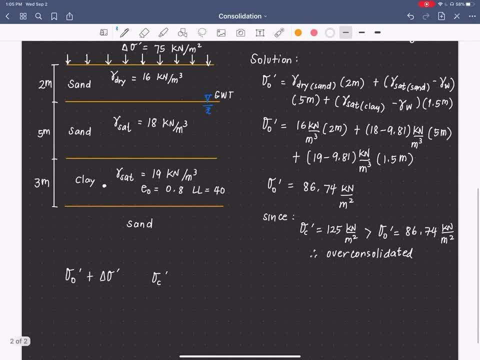 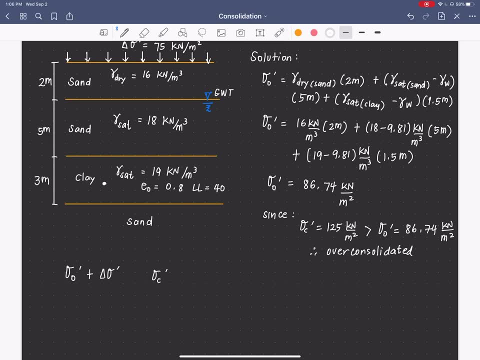 equal or less than so that we could identify which formula to use in calculating the primary consolidation. so our effective stress is 86.75 plus our given surcharge, or Delta Sigma, is 75, while our preconsolidation stress is 125. so if you get the sum of this, this is 161 point 74 and obviously 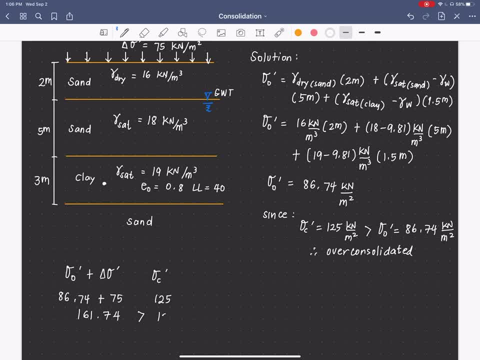 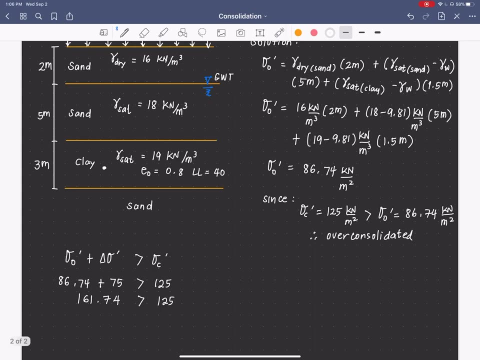 greater than 125, so our effective stress plus surcharge is greater than our preconsolidation pressure. so in this case the formula that we have to use is this one. the primary settlement is equal to C sub s H over 1, plus a civil log off Sigma sub C prime divided by Sigma sub o prime plus. 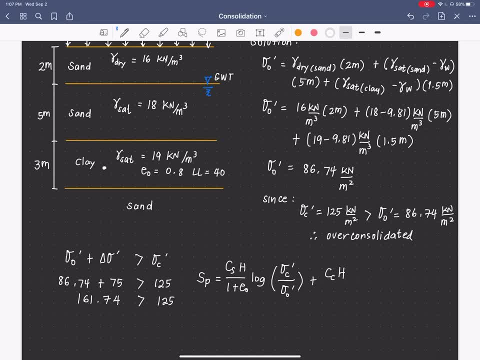 C sub C H over 1 plus a sub o or a sub not log off over 1 plus a civil log off. Sigma sub C prime divided by Sigma sub o prime, plus the effective stress plus the surcharge divided by the preconsolidation pressure. 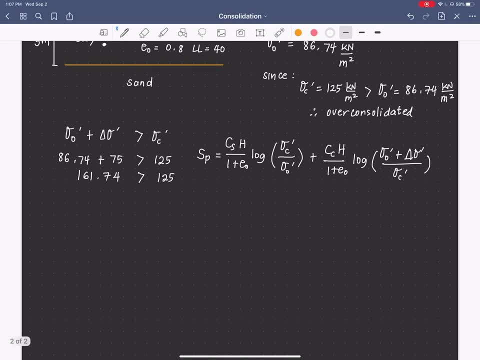 Okay. so, having this formula, let us check if all the parameters are available. C-sub-S is given to be 1 sixth of C-sub-C, So here we have to calculate for C-sub-C, so we can compute for C-sub-S. 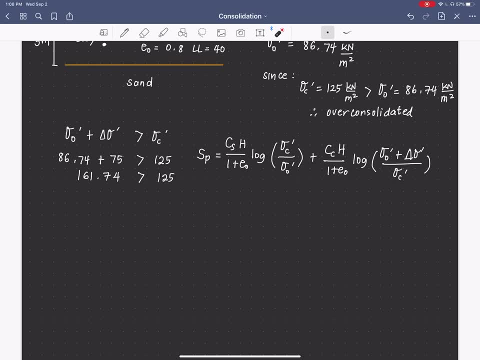 The thickness of the clay layer is known. E-sub-O or the in-situ void ratio is known. The, The, The preconsolidation pressure, is already known, Overburden pressure is known And the delta sigma is known. So all we have to compute is 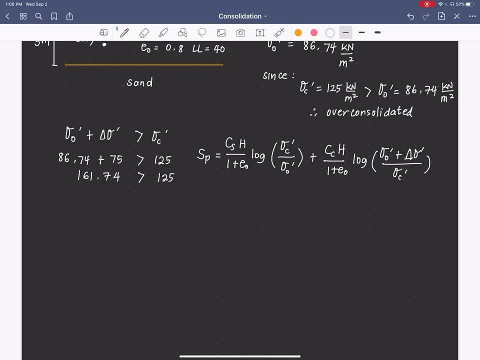 E-sub-O. So let me write here, I'm sorry- the C-sub-C. Okay, It is assumed that the soil is undisturbed And we can use the Skempton's formula for C-sub-C, which is 0.009.. 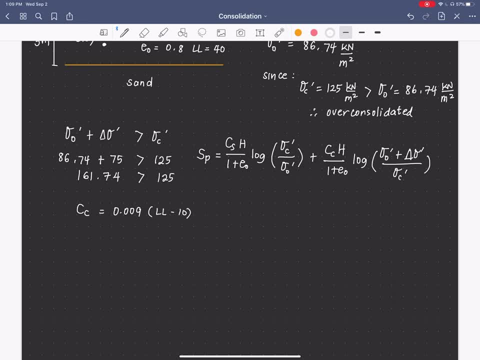 Liquid limit minus 10.. Our liquid limit is given to be 40, right Minus 10.. So our C-sub-C value is 0.27.. So from there we can solve for the soil index, which is 1 over 6 of our C-sub-C. 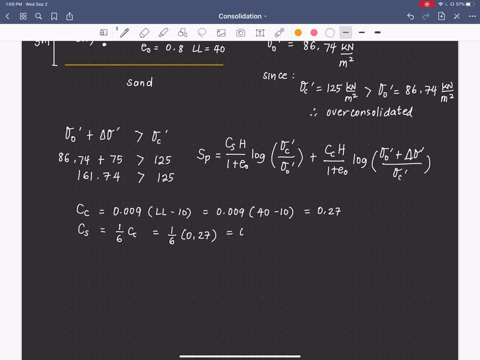 And that will give us 0.045., 0.045., 0.045., 0.045., 0.045., 0.045. 0.045.. So we have values of all the parameters, So we can now plug in these values to solve for our primary settlement.